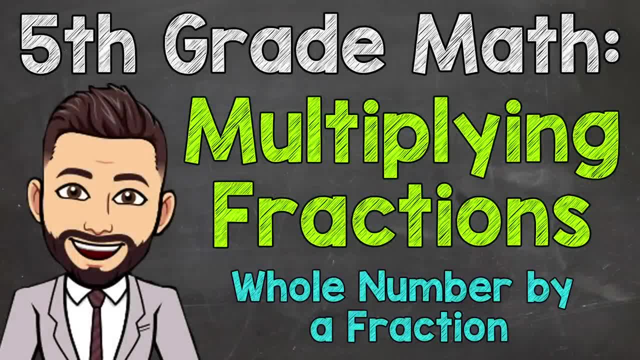 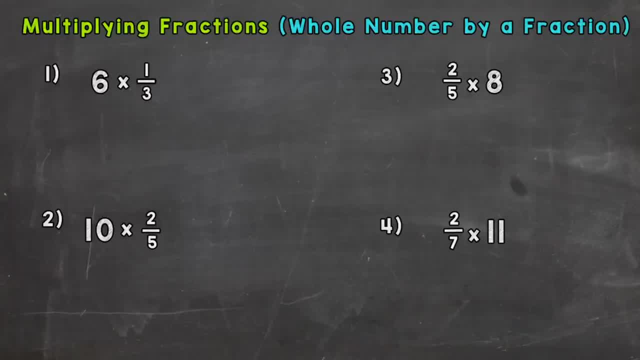 Welcome to 5th Grade Math with Mr J. In this video we are going to be covering multiplying fractions by a whole number. So, as you can see, there are four problems on your screen. We're going to go through these four problems together and hopefully, by the end of the four problems you have this down. 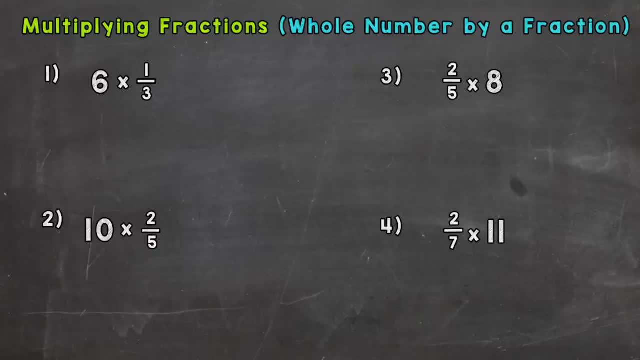 My suggestion would be to write these out with me and if at any point you feel confident enough to try a couple on your own, feel free to press pause and then, when you're ready, press play and check the remaining problems with how I do those problems If you want to do all four with me. 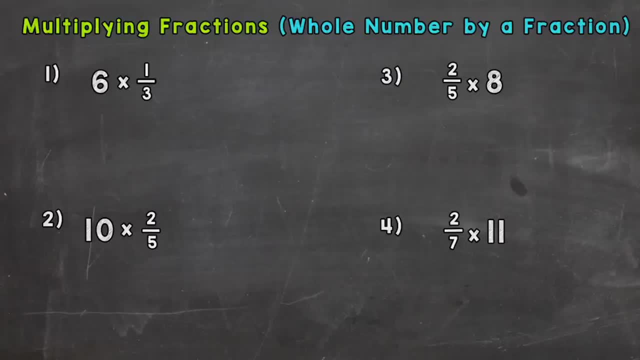 that's fine as well. So let's jump right in to number one. and we have six times one-third. So whenever we're multiplying a whole number by a fraction, the first thing we want to do is take the whole number and make it into a fraction, And all you have to do 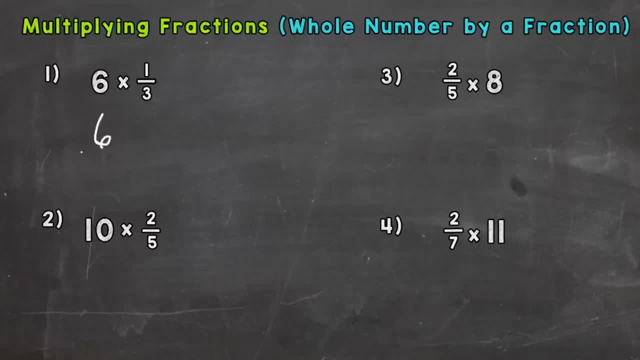 for that is, multiply the whole number by a fraction, And that's what we're going to do, For that is, you need to put the whole number over one. Now we have a numerator and a denominator- and then bring down the rest of your problem. 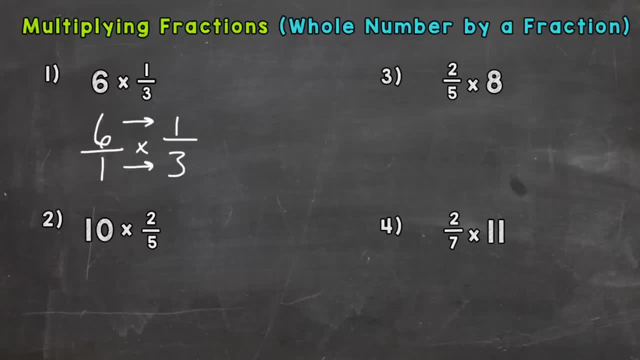 So when we multiply fractions, all we do is go straight across Numerator, times numerator, denominator, times denominator. So six times one is six and one times three is three, So we get to six-thirds. Now that's an improper fraction, meaning the numerator or top number. 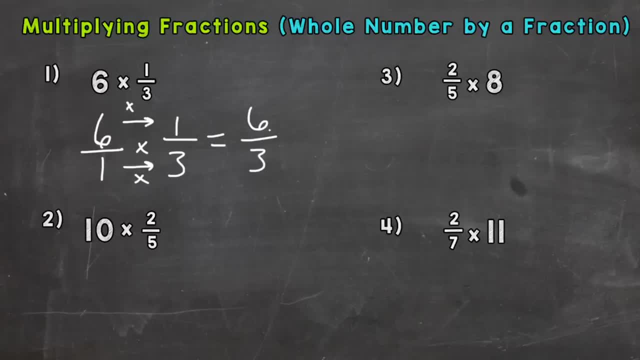 is greater than the denominator. So what we do is we divide the numerator by the denominator, So six divided by three, and that's going to give us a whole number answer. So how many whole groups of three can we pull out of six? And the answer to that is two. Is there a remainder? 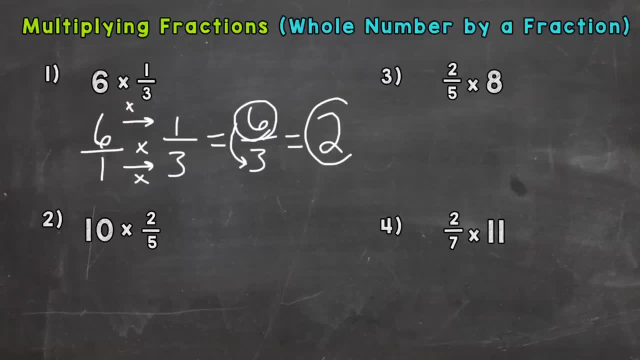 To that problem? No, So we are done. The answer is two. Now let's take a look at how the answer relates to our original problem. So we started with six times one-third and we ended up with an answer of two. Now, normally when you multiply whole numbers, 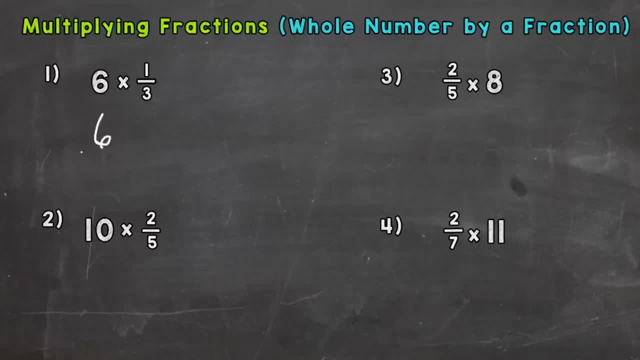 for that is, multiply the whole number by a fraction, And that's what we're going to do, For that is, you need to put the whole number over one. Now we have a numerator and a denominator- and then bring down the rest of your problem. 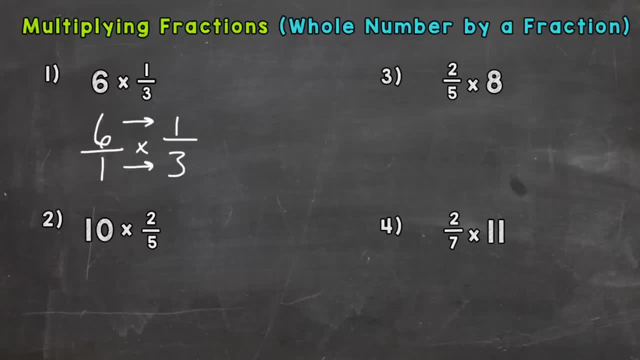 So when we multiply fractions, all we do is go straight across Numerator, times numerator, denominator, times denominator. So six times one is six and one times three is three, So we get to six-thirds. Now that's an improper fraction, meaning the numerator or top number. 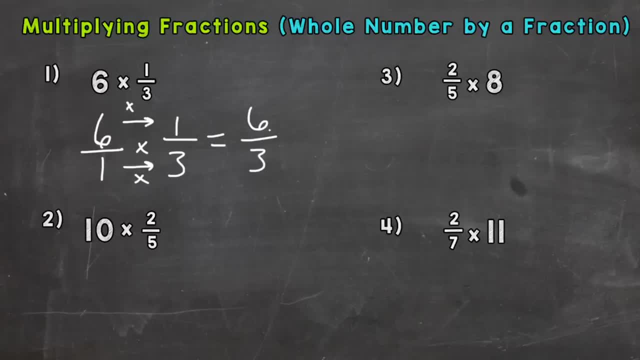 is greater than the denominator. So what we do is we divide the numerator by the denominator, So six divided by three, and that's going to give us a whole number answer. So how many whole groups of three can we pull out of six? And the answer to that is two. Is there a remainder? 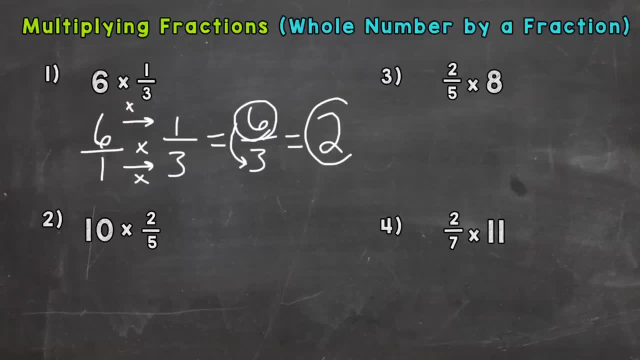 To that problem? No, So we are done. The answer is two. Now let's take a look at how the answer relates to our original problem. So we started with six times one-third and we ended up with an answer of two. Now, normally when you multiply whole numbers, 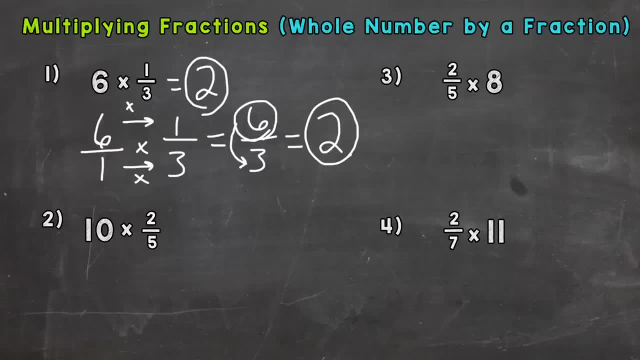 your answer is going to be greater than the numbers you started with, But since we multiply by a number or a fraction, less than one whole, our answer actually got smaller in value than the six that we started with. So even though we multiplied, our answer got smaller than. 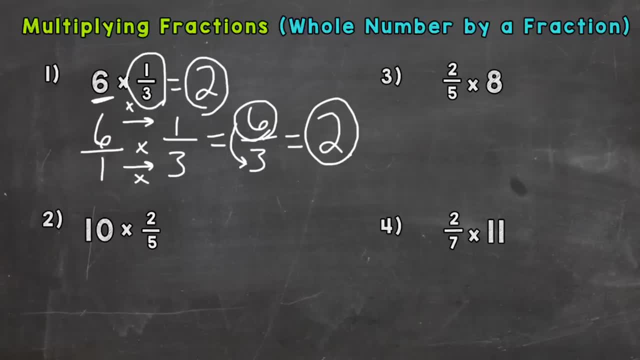 what we started with, because we multiplied by a number that was less than one whole. So let's take a look at number two And, to go off what we were just talking about, we're multiplying ten by two-fifths- A number or fraction that's less than a whole, So our answer is actually going to be less than ten. 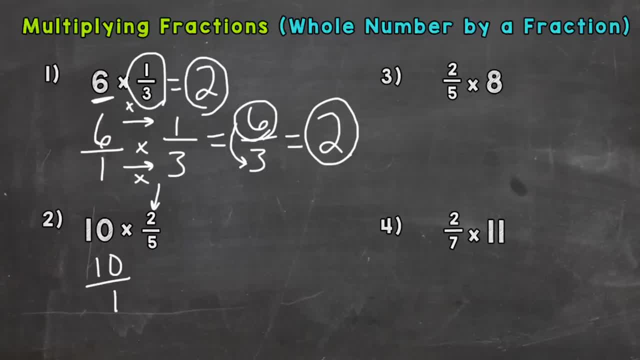 So put your whole number over one, Bring everything else down and now we multiply. Ten times two is twenty. One times five is five. So we have an improper fraction here. We don't want to leave our answers as improper fractions, So we divide the numerator. 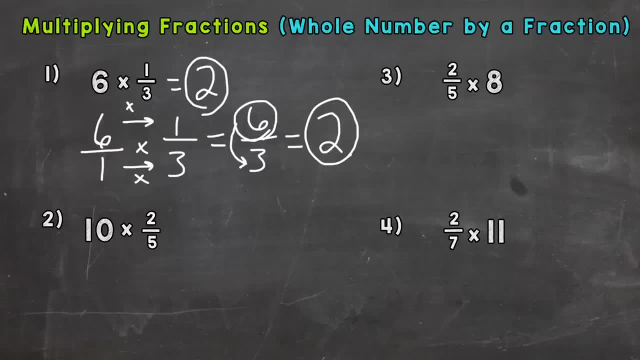 your answer is going to be greater than the numbers you started with, But since we multiply by a number or a fraction, less than one whole, our answer actually got smaller in value than the six that we started with. So even though we multiplied, our answer got smaller than. 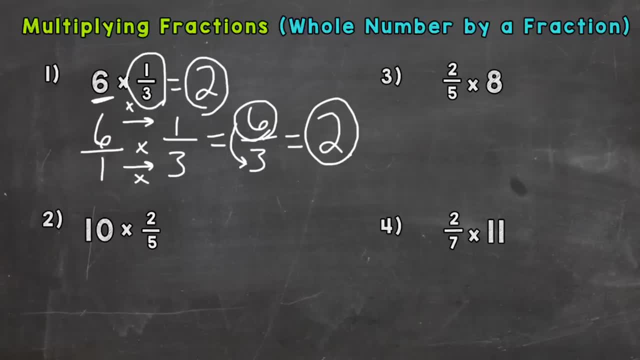 what we started with, because we multiplied by a number that was less than one whole. So let's take a look at number two And, to go off what we were just talking about, we're multiplying ten by two-fifths- A number or fraction that's less than a whole, So our answer is actually going to be less than ten. 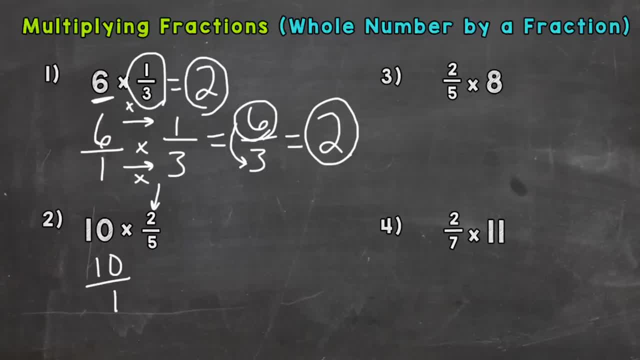 So put your whole number over one, Bring everything else down and now we multiply. Ten times two is twenty. One times five is five. So we have an improper fraction here. We don't want to leave our answers as improper fractions, So we divide the numerator. 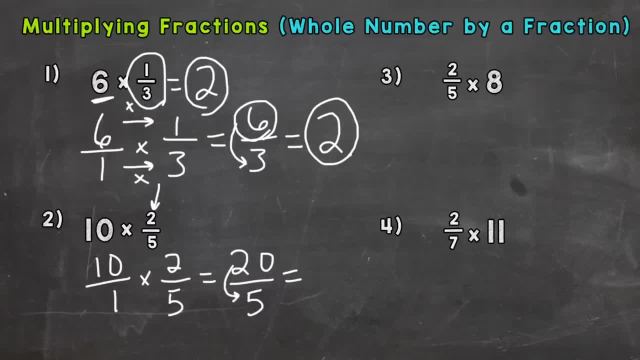 the top number by the denominator. So twenty divided by five. How many whole groups of five can we pull out of twenty? Well, four, Any remainder or anything left over? No, So our final answer is four. Let's go to number three, Two-fifths times, put eight over one, So we have a top and a bottom. 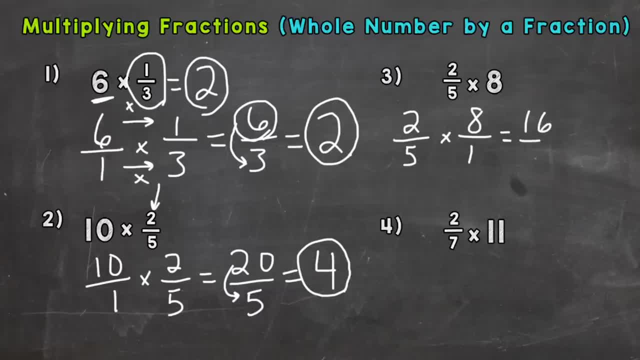 cross 2 times 8, 16.. And 5 times 1 is 5.. Again, we have an improper fraction. so we need to do 16 divided by 5.. How many whole groups of 5 can we pull out of 16?? And the answer to that is 3.. 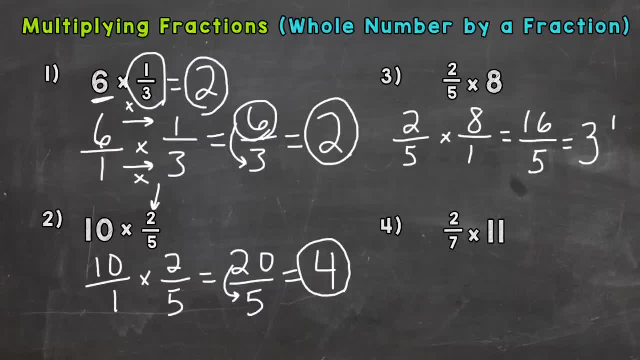 But we have 1 left over, right 16 divided by 5, we get 3 with a remainder 1.. So that remainder is a numerator here, and then we keep the denominator the same, So 3 and 1. fifth, 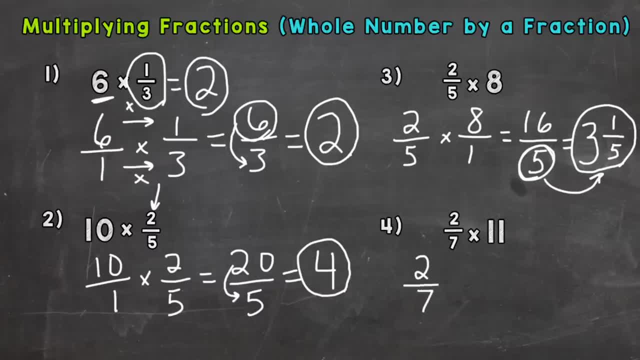 Number 4, 2 sevenths times 11.. Put it over: 1. 2 times 11 is 22.. 7 times 1 is 7.. So again an improper fraction. So we need to do 22 divided by 7, which is 3, and we get a remainder 1, and keep the denominator. 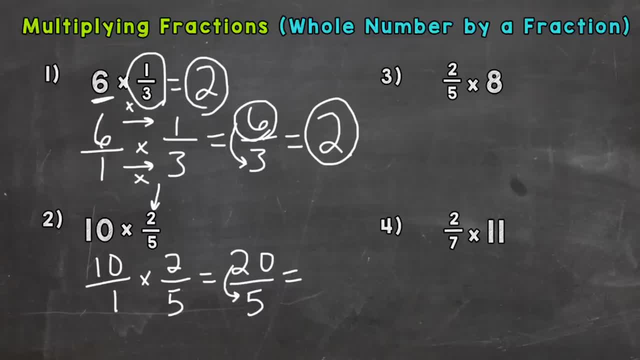 the top number by the denominator. So twenty divided by five. How many whole groups of five can we pull out of twenty? Well, four, Any remainder or anything left over? No, So our final answer is four. Let's go to number three, Two-fifths times, put eight over one, so we have a top and a bottom, And then multiply straight across the top. We can see that the numerator is four and then we divide by two-fifths. Two-fifths times, we get eight over one. So we have a top and a bottom And then multiply straight across the top. So we have a top and a bottom And then multiply straight across the top And then multiply straight across the top. 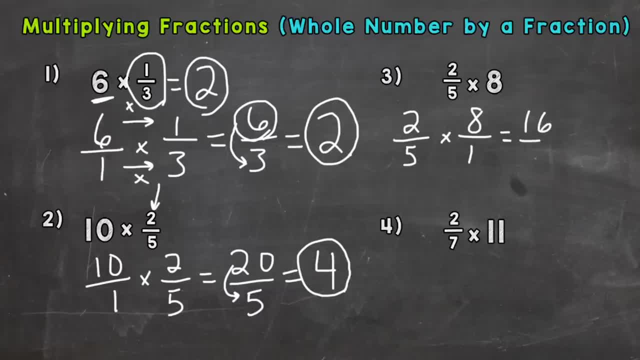 cross 2 times 8, 16.. And 5 times 1 is 5.. Again, we have an improper fraction. so we need to do 16 divided by 5.. How many whole groups of 5 can we pull out of 16?? And the answer to that is 3.. 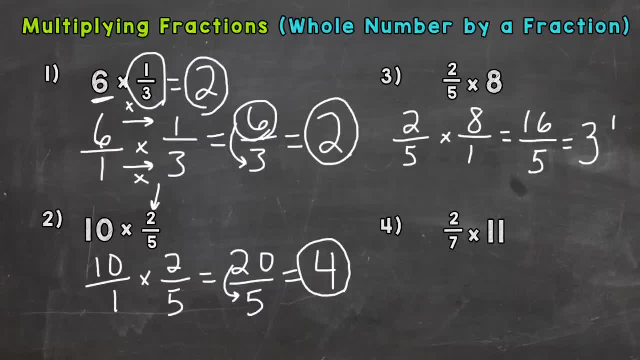 But we have 1 left over, right 16 divided by 5, we get 3 with a remainder 1.. So that remainder is a numerator here, and then we keep the denominator the same, So 3 and 1. fifth, 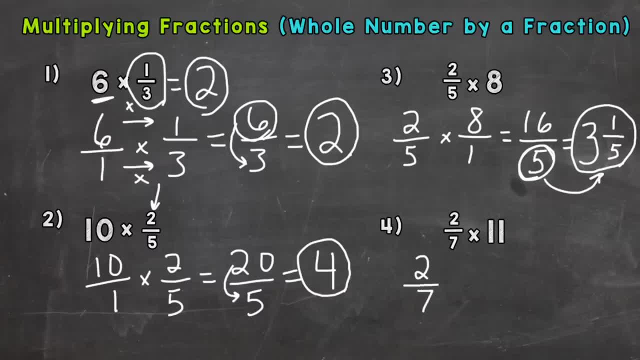 Number 4, 2 sevenths times 11.. Put it over: 1. 2 times 11 is 22.. 7 times 1 is 7.. So again an improper fraction. So we need to do 22 divided by 7, which is 3, and we get a remainder 1, and keep the denominator. 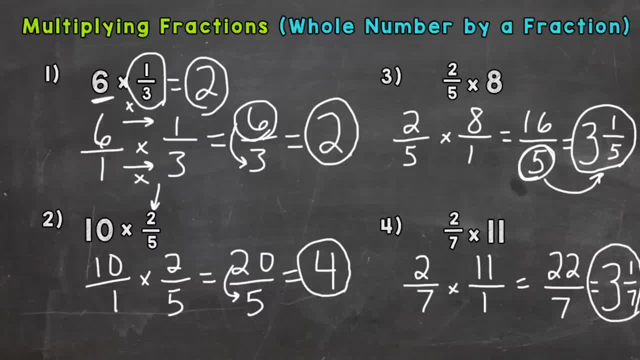 the same. So 3 and 1. seventh, Again, we did 22 divided by 7, and got 3 wholes with a remainder 1 here, and we keep the denominator the same. So there you have it, multiplying fractions. 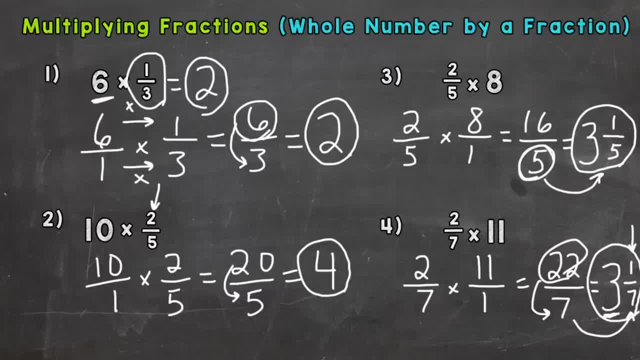 a whole number by a fraction. Just remember: you put your whole number over 1, and then you have a numerator and a denominator and you can multiply straight across. Thanks so much for watching and until next time.